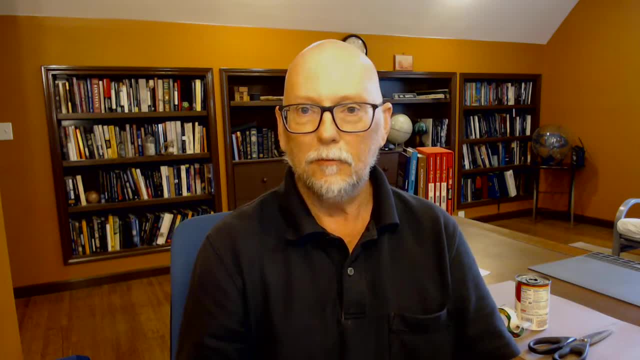 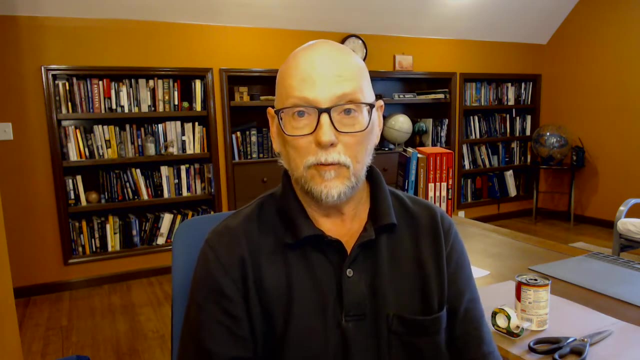 how many stars are there in the sky? How many can you see? The traditional number for this is 6,000, but that involves pristine dark skies visible to the naked human eye. Most of us don't have pristine dark skies. We live in urban or suburban environments where light pollution affects how 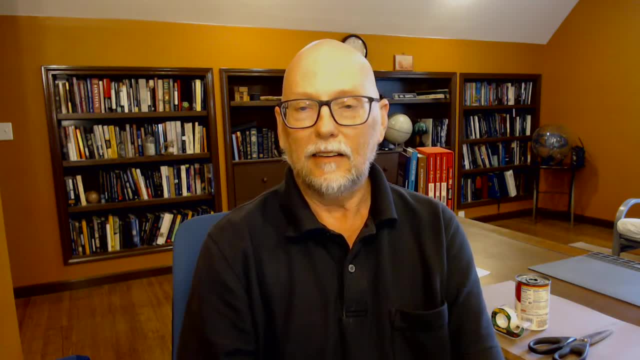 much we can see: Light pollution, light that shines at night in inappropriate places where we don't need to see. this affects not just human sleep, but also nocturnal animals, insects. There's all kinds of environmental impacts, not to mention the 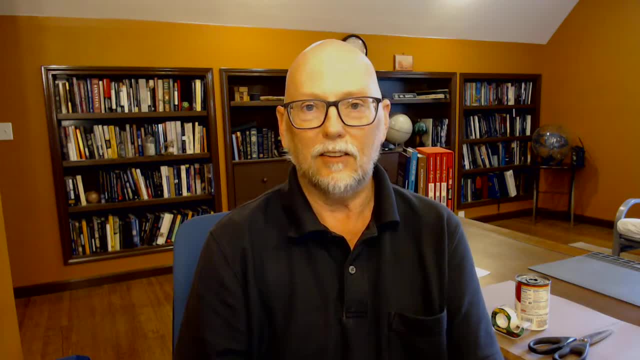 environmental impact of the environment. We live in a world where there's a lot of pollution. We live in a world where there's a lot of pollution. We live in a world where there's a lot of energy we waste shining up lights into space. It's really quite shocking. One of the ways students 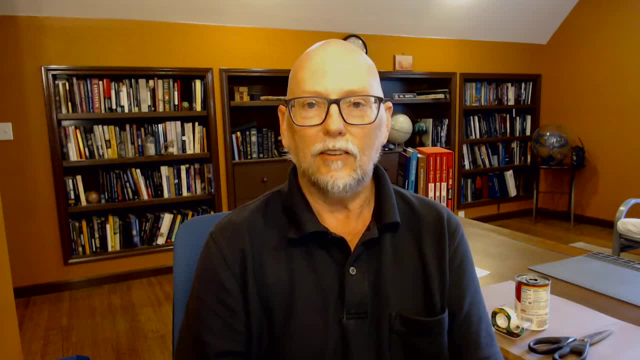 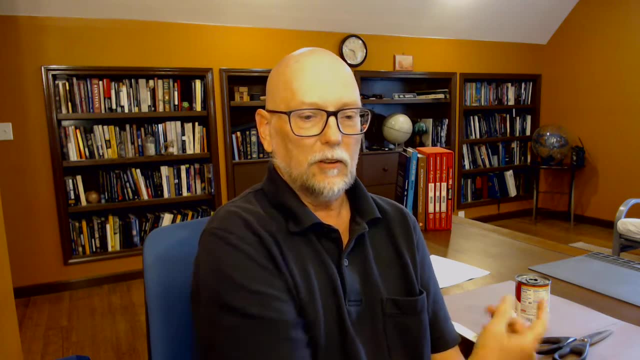 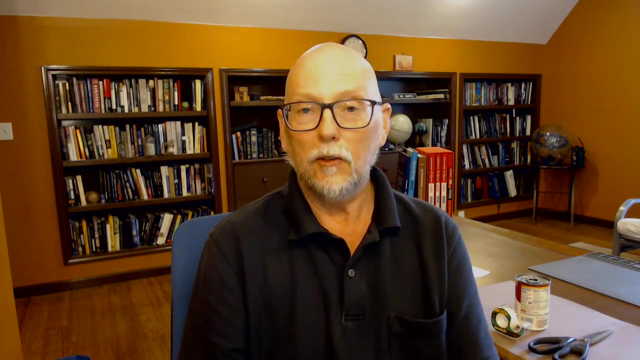 can get involved with this is to make a light pollution map, And to do that, we're going to use some simple methods with inexpensive materials. We'll use a can of soup, some scissors, some construction paper and tape and we're going to count the stars in the sky. Now you might ask: 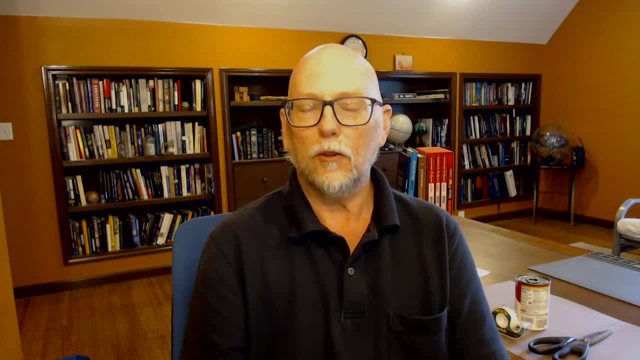 how can we count all the stars in the sky? The answer is quite simple. It's called statistical sampling. If we take a small section of the sky, what we can see through a rolled up paper tube, and we multiply it out, we know what fraction of the sky we're looking at. 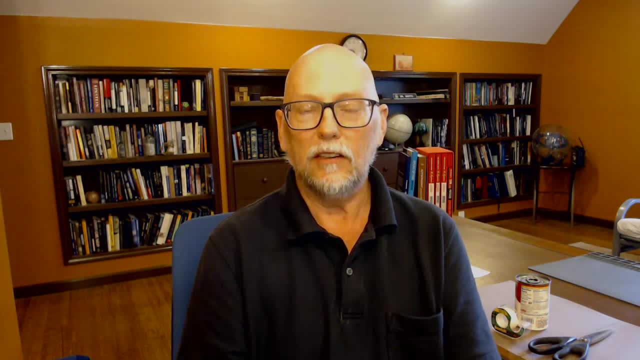 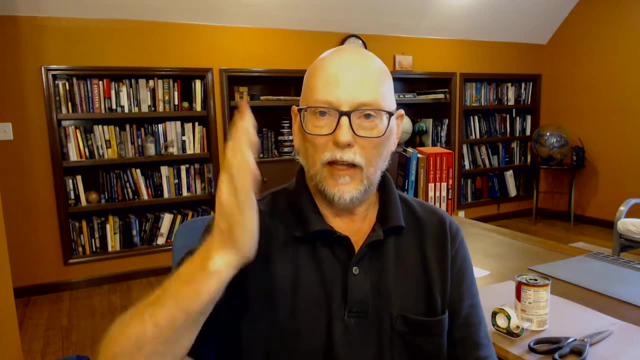 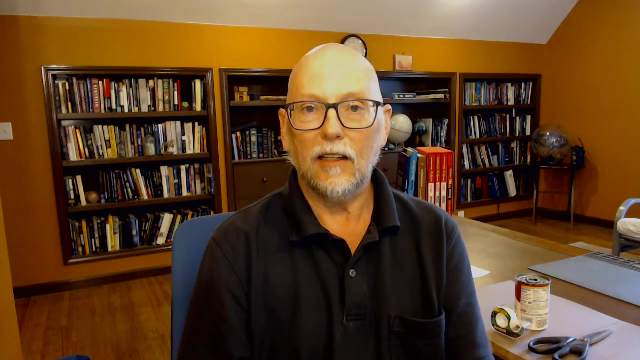 then we can find out how many stars we can see from our location. Moreover, doing this in multiple directions and multiple angles off the horizon, we can make for ourselves a light pollution map. We'll see how in a minute, but let's take a few seconds and see how it works. 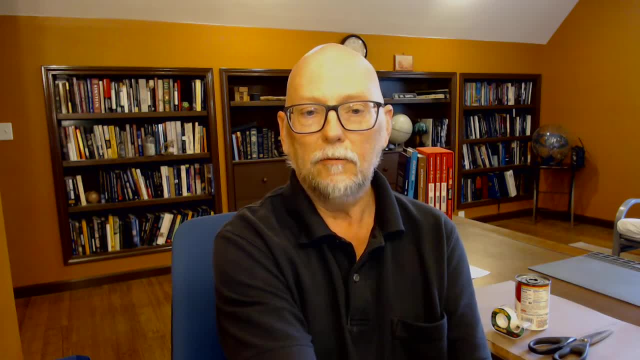 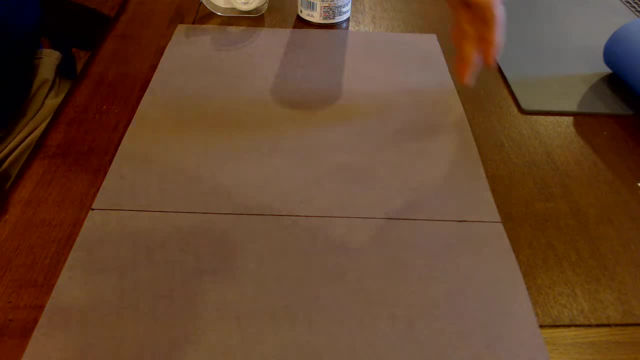 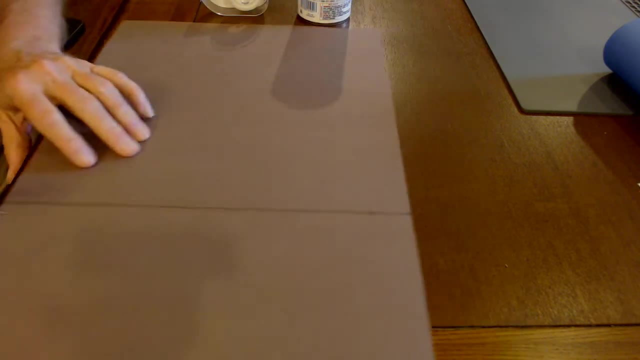 Let's see how we use our materials for today. Here we are. We've taken a regular sheet of construction paper- and most commercial construction paper is about 12 by 18 inches and it makes it very easy to make a 30 centimeter square. And we're going to take our 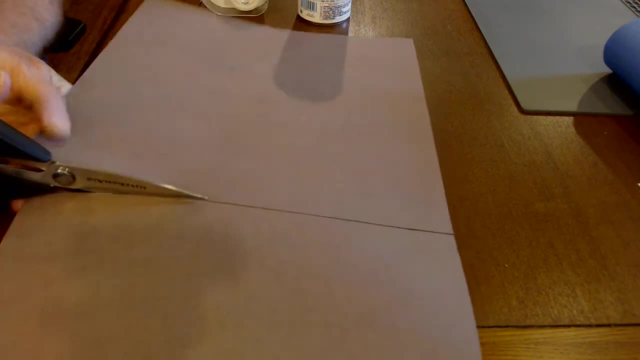 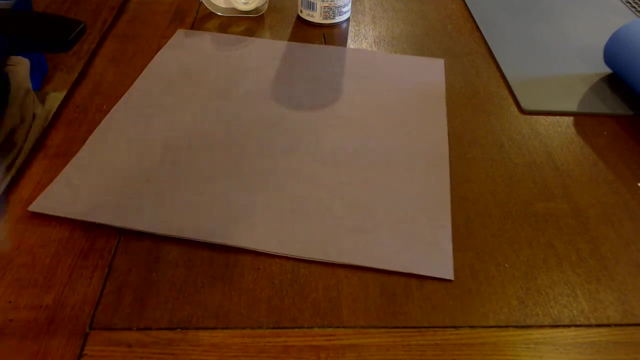 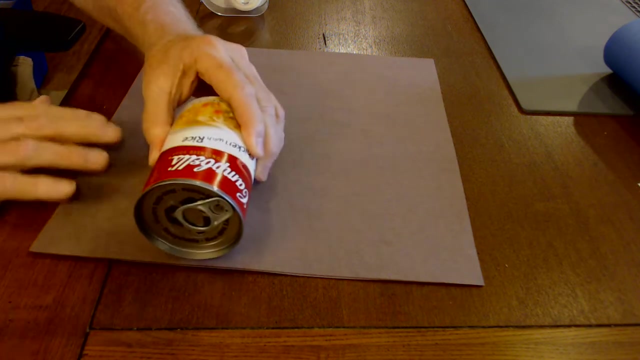 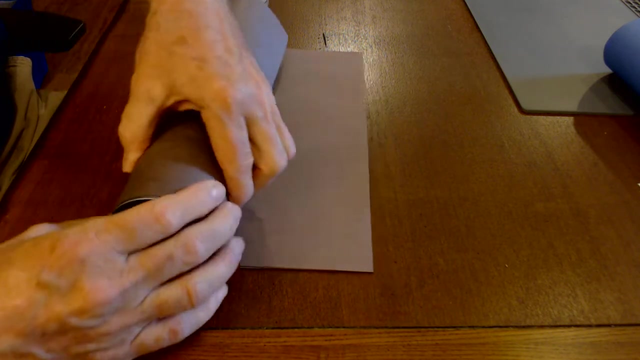 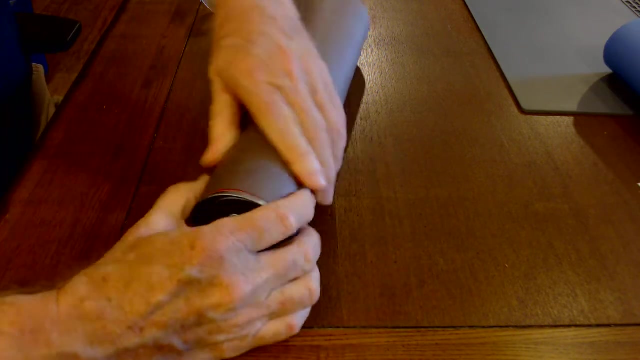 scissors and we've measured this out and we're simply going to cut out our 30 centimeter square. Doesn't have to be very perfect. There we go, And now what we're going to do is we're going to use a regular can of soup here And I'm going to go ahead and take and roll the paper around in it, And I'm going to try to be careful to make it straight, Although, again, perfection isn't necessary. 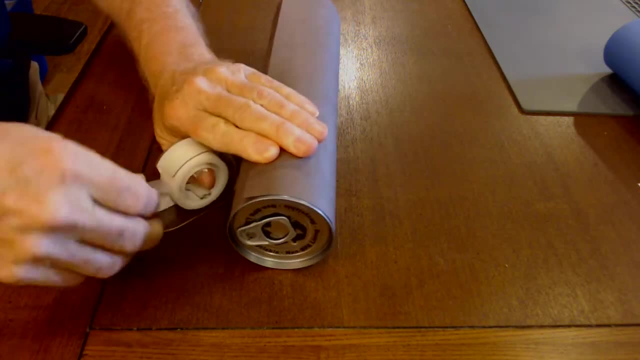 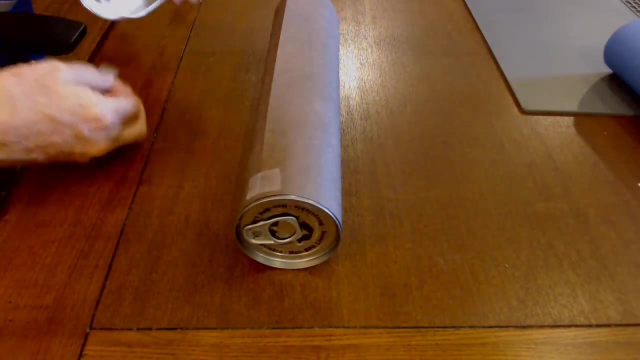 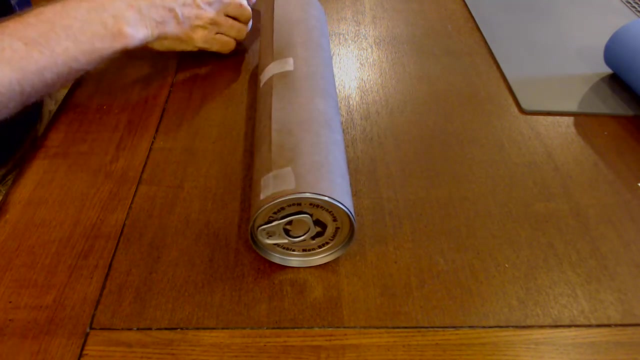 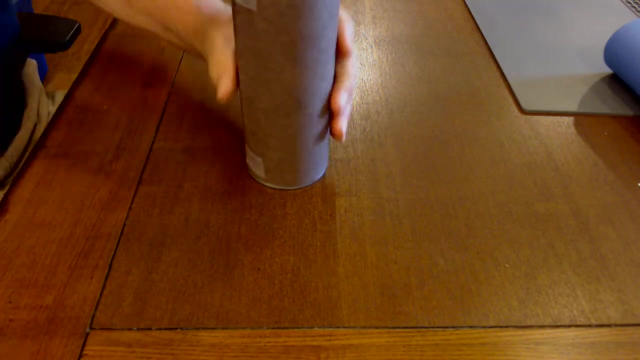 It just needs to be relatively neat. I'm going to go ahead and tape my paper together. Dark colored paper is preferred here, friends. Light colored paper can actually reflect light down to the observer and interfere with the count of stars. But I've got it taped at the top, middle and bottom. One, two, three And then bingo, the can of soup comes out and we have a soup. 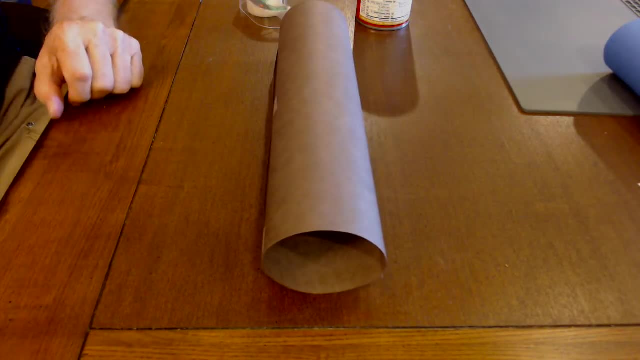 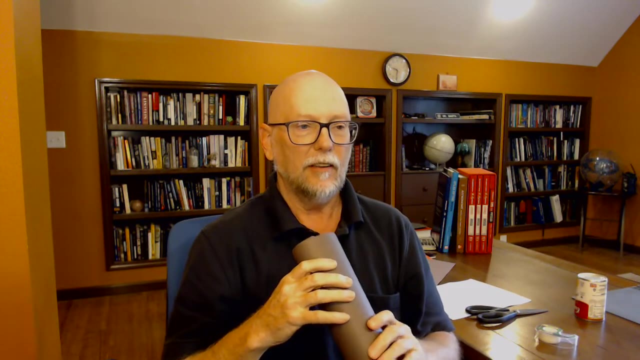 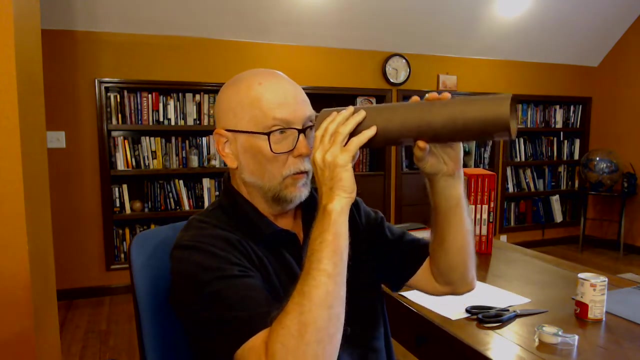 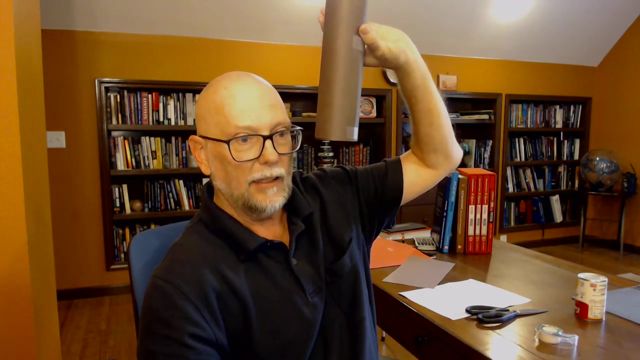 And we have our sighting tube. Now we'll show you how this activity works Now that we have our sighting tube. the entire idea here is that we're going to have our students look through horizontally at the horizon. That's our zero degree angle. We're going to raise it up 30 degrees, 60 degrees And finally we'll be looking through straight at 90 degrees. The idea is that we're taking the sky. 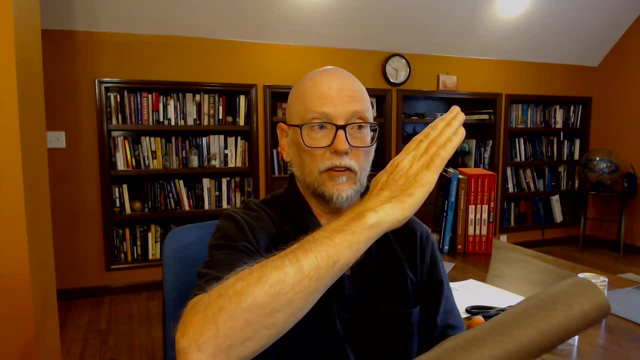 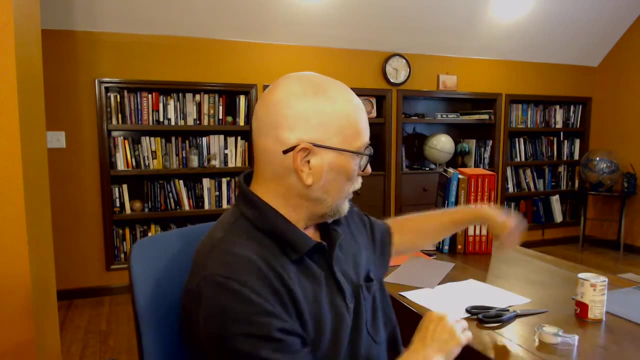 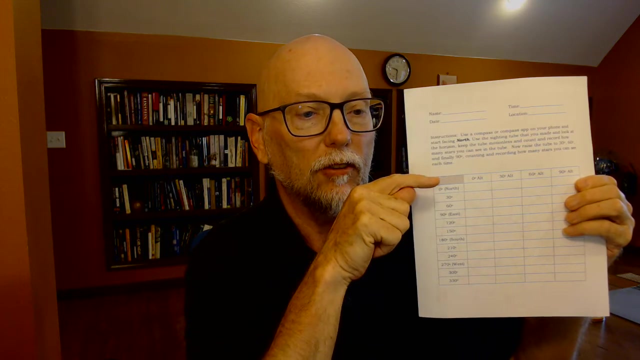 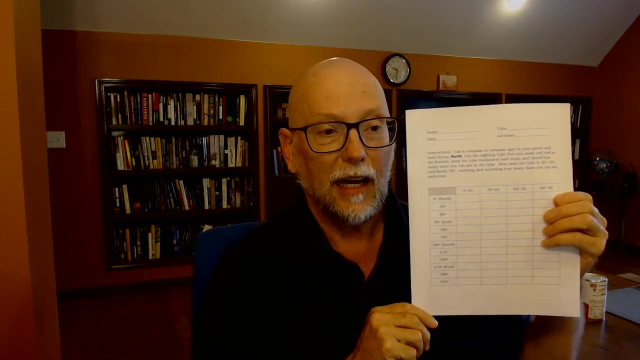 One third of the way, 30 degrees, two thirds, 60 degrees, straight up, 90 degrees, And we're going to do this for 12 directions. We'll end up with a data sheet here- And, yes, I have a data sheet for you- And the data sheet shows here's our azimuth or compass directions, And we go zero through 330.. These are basically the hours of the clock. So even if you don't have a compass or a compass app on a phone, you're going to have a compass app. 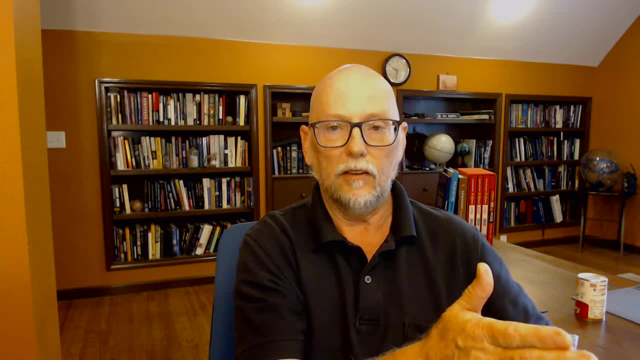 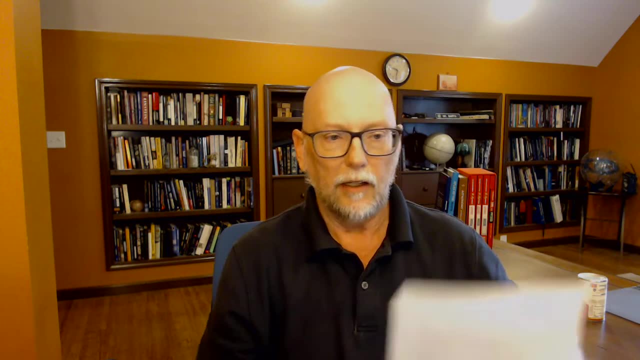 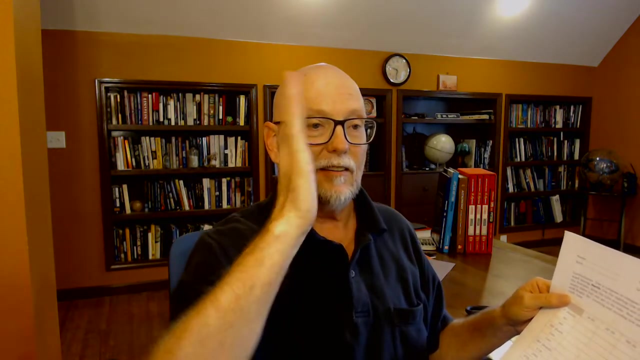 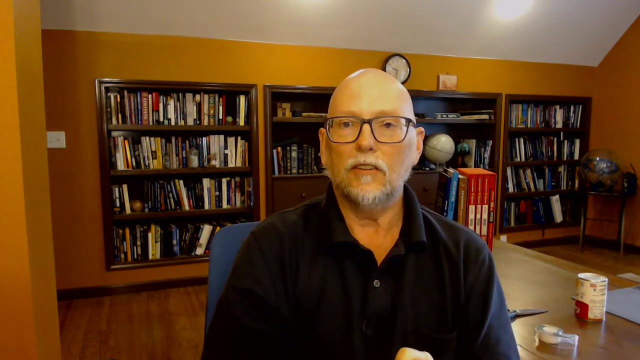 And you can think of a clock. Here's: 12 o'clock is zero, One o'clock is 30 degrees, Two o'clock is 60 degrees, and so on, And you can go ahead and get all of your data recorded in each direction, for zero, 30,, 60, and 90 degrees. Now what's interesting- and I don't even tell my students this, of course- is that 90 degrees serves as a control for our experiment. 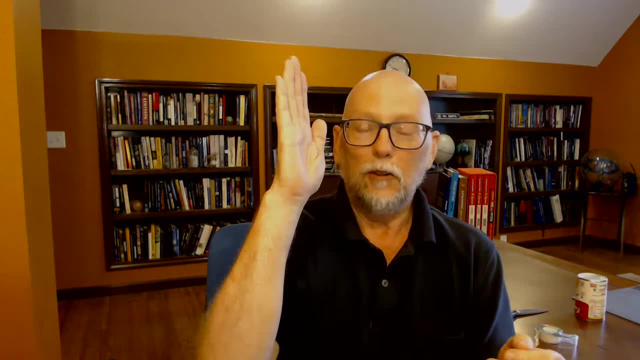 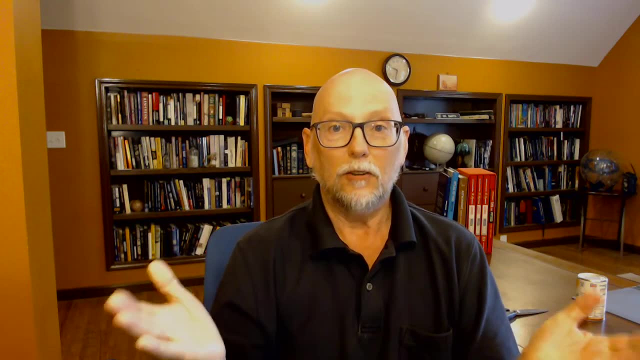 If, no matter what direction you're looking at, you're going to have a compass. If, no matter what direction you're facing, if you point the tube straight up and you're standing in one place and you count, then each of the 90 degree counts should be pretty close to the same. 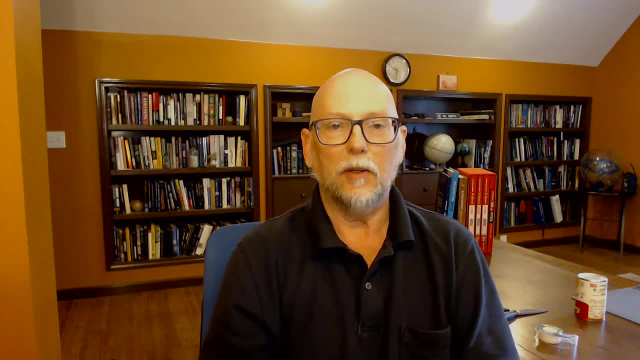 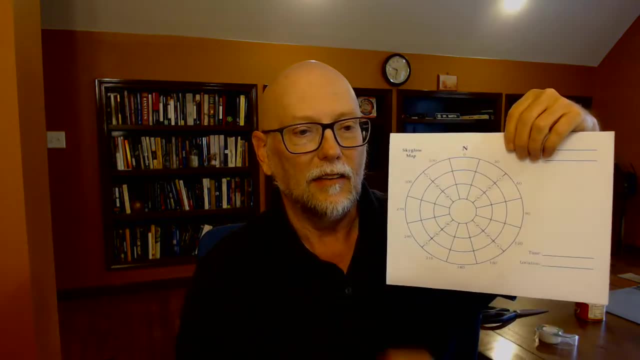 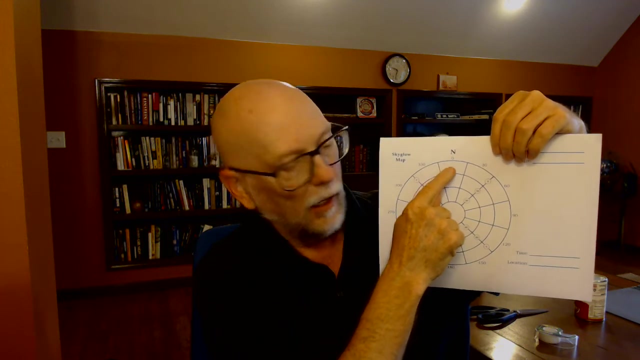 They should agree with each other. This tells us about sampling, accuracy and experimental methodology. Now, when we're done gathering data, I have a lovely chart here which shows all of our directions, And we have rings for horizon, zero, degrees, 30,, 60, and we can average all of our 90 degree numbers and place them here. 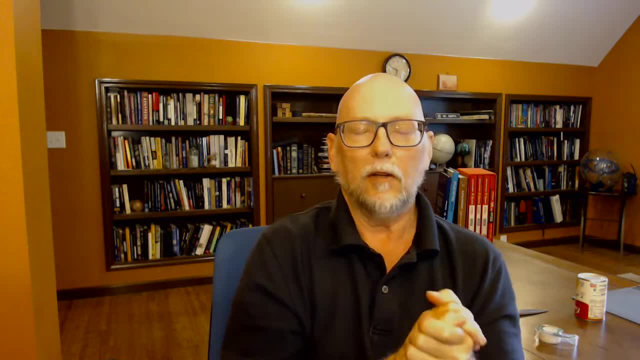 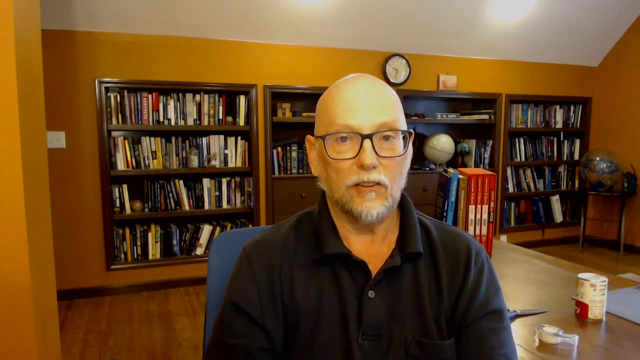 Now, once students do this, when they look at the map, it should become clear to them that some areas show more stars than others. The areas, of course, that show less stars indicate more light pollution, interfering with their ability to see and count stars in the sky. 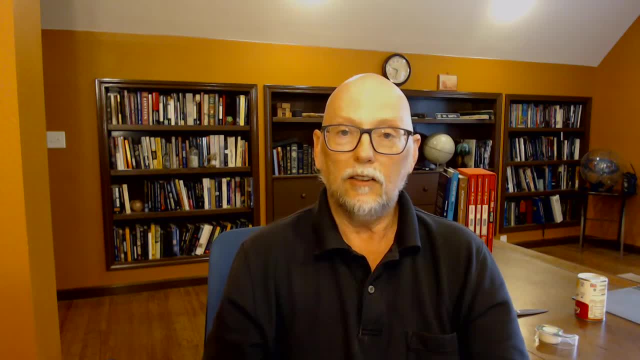 This is a fascinating exercise and we can use it as a basis later If we're doing outdoor observations for planning. oh gee, we want to observe Saturn and Jupiter this summer while they're in the sky, in opposition and very bright. Well, obviously, we're going to get the best views of these things if we're observing in areas of low light pollution. 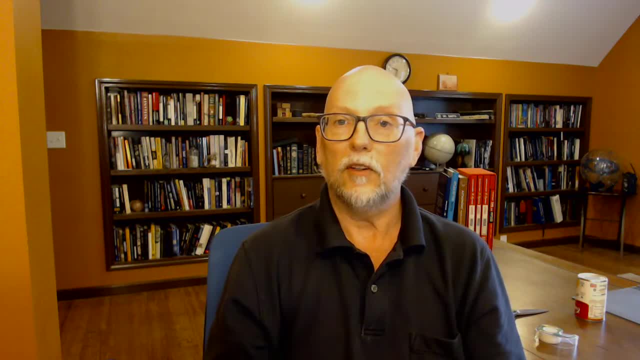 And our map can tell us this. Furthermore, this is an inexpensive and fun activity. It translates very well if you have students working in a remote hybrid classroom situation Or if you want to give students an activity to take home and try on their own. 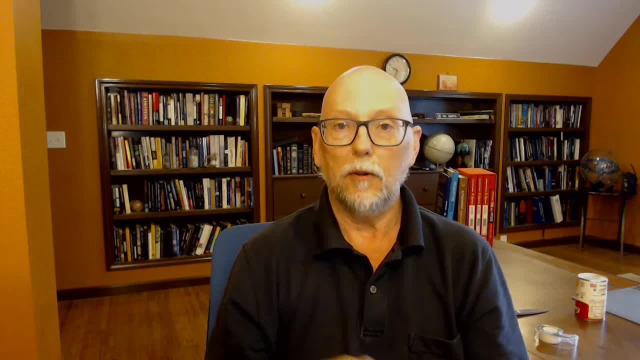 Furthermore, if you're having a back-to-school night coming up, it's always great to have your students show off how smart they are and what fascinating things they've done, And this project with a light pollution map makes a great back-to-school night exhibit.